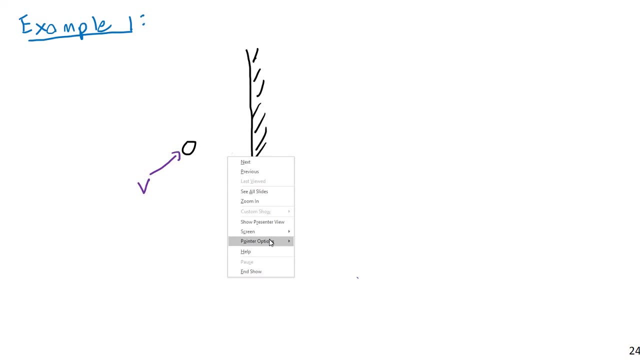 Simply v here, velocity v, and it's going to follow a path something like this: It will ricochet, And I know from basic physics that if there's only one object striking a horizontal wall, it will rebound. it will rebound with the same angle. 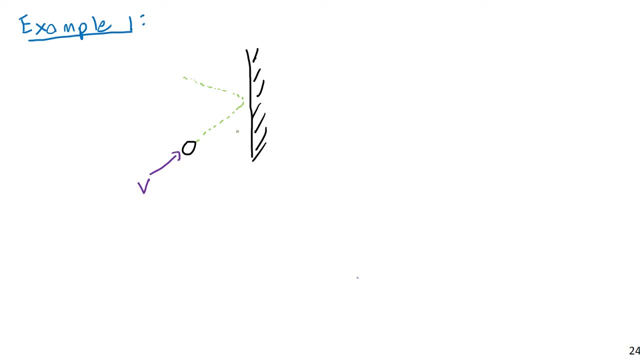 Um, anyway, then let's say, Let's say that the um, the angle here, the angle of impact is 30 degrees here. Uh, so it forms an angle of 30 degrees And actually, well, I don't want to say that that will rebound at the same angle. 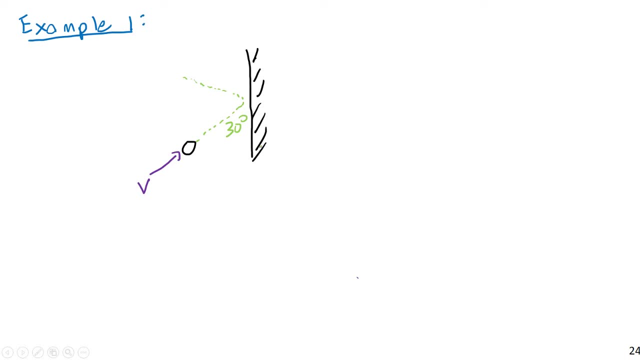 So, um, I actually don't want to say that It may not. Um, so let's um resolve this and see how this will end up. So, actually, in this case, it may not end up with that. That would be for a perfectly elastic collision. 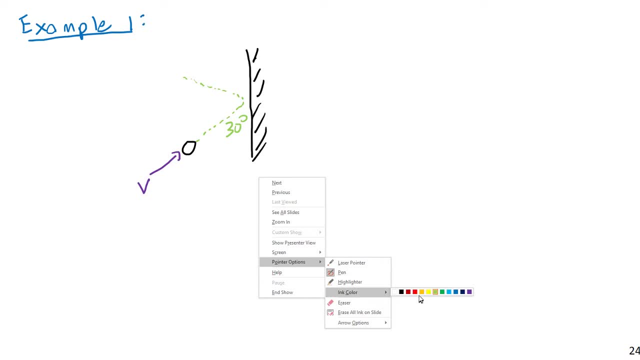 I don't necessarily want to say that That would be, uh say, a bouncy ball. I mean something like a I don't know. a good example would be light, Uh, a particle of light, a photon, striking the surface and reflecting off a mirror or something. 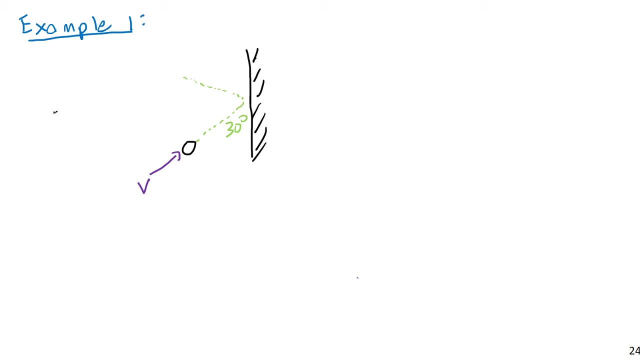 Okay, And also I will be told that the coefficient of restitution is 0.90.. And I wish to find, Uh, I wish to find the magnitude and direction- And I will label this as given here- And I wish to find magnitude and direction of the uh reflected ball. 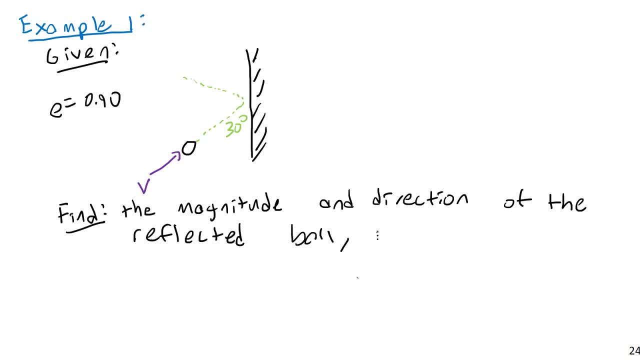 In terms of V. So in terms of V, Uh, in terms of V, All right, So let's get this here Now. and also, this is a frictionless surface here, Frictionless vertical surface, Okay. 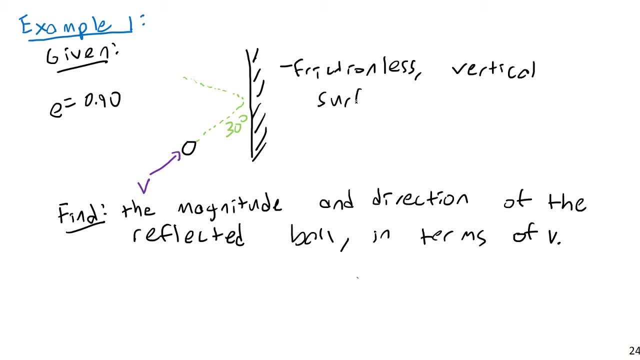 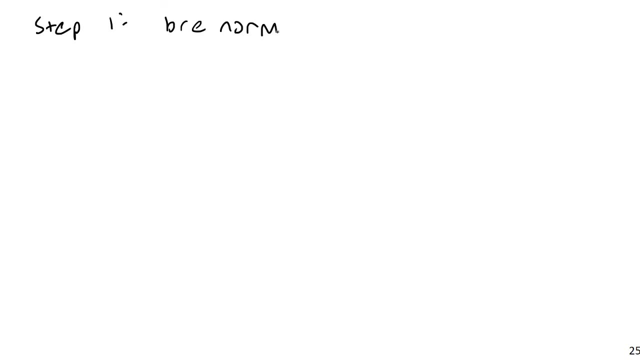 um, normally tangential components, uh relative to the wall And tangential components relative to the wall, All of these would be also could also be considered vertical and horizontal in this case. Uh, I should say, break uh velocity, the wall velocity, into normal and 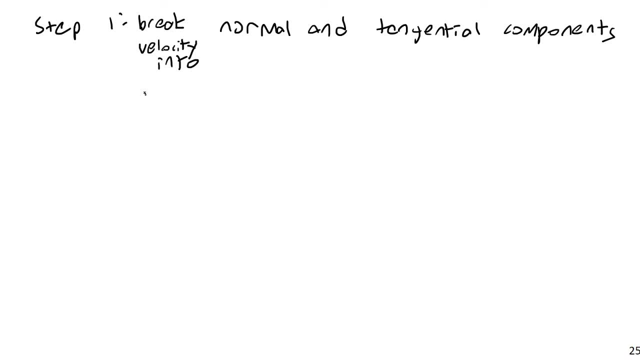 tangential components. So basically, let me draw this out here: The ball coming in will have a um here, And I could do this in vertical and horizontal. However, I don't want to necessarily do that because I want to get in the habit of realizing. 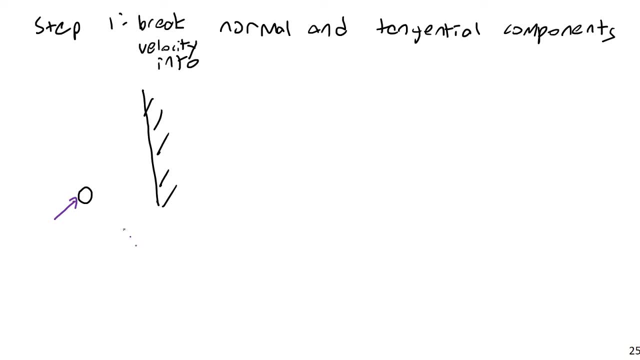 that a lot of our components break down in terms of normal and tangential planes. So I could actually, in this case, normal tangential will actually be vertical and horizontal, but uh, or actually uh, vice versa. But I do want to just sort of get in the habit. 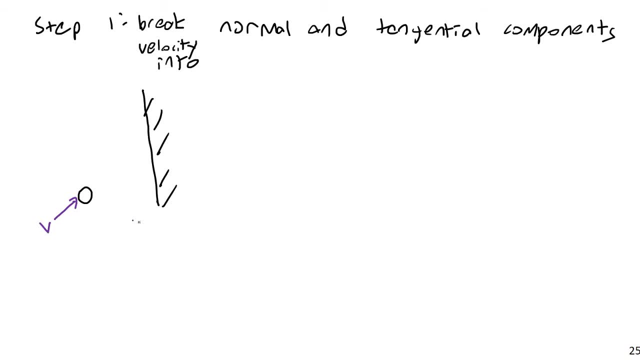 of doing this. So this is our velocity, um, initial, and I can just say v our initial velocity, and this will have components uh v tangential, so tangent to the surface here, and then component uh v n v normal And 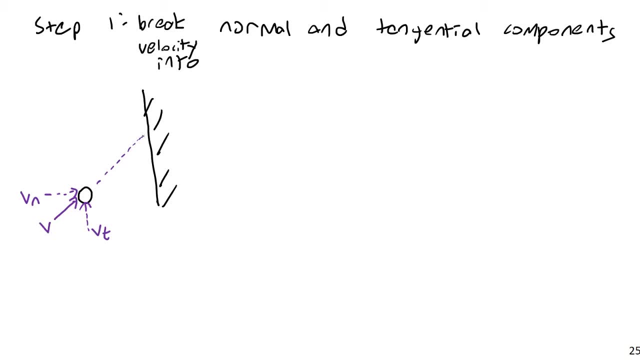 then this thing will rebound and after it rebounds the ball will be over here somewhere and it will have components, also tangential, and vertical and and normal. It will have components. uh, actually I could use the same color. It will have components v, t. 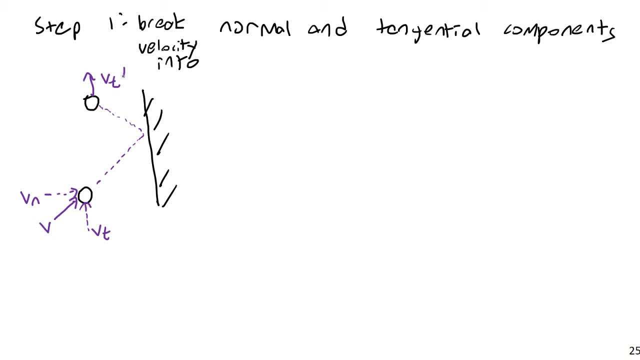 prime and v n prime. I don't know the exact um magnitudes of these, but I can go ahead and assume that the normal component is going to be this: the v n prime. So it's going to be the, the v n prime, And this will be the sum of all the components. This is the. this. 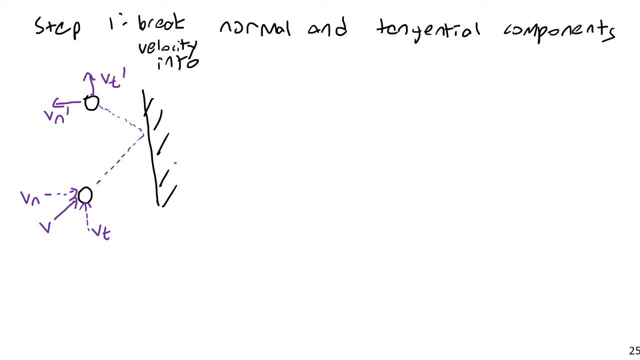 v n prime. I don't have the exact um magnitudes of these, but I can go ahead and assume that will be going to the left and the vertical and the tangential component will be going upward. So let's go ahead and do this. Okay, so we're solving, and so I actually get the initial. 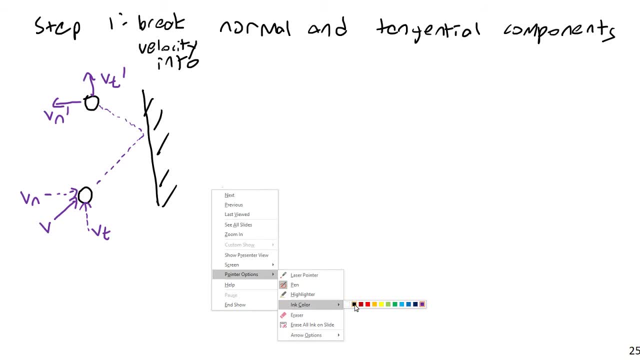 components. So this is actually not bad. this is just basic vector algebra, this is just trigonometry. So vn here is going to be v cosine. 30 degrees is equal to 0.866 v. 0.866 v and v tangential is going to be v sine of 30 degrees. 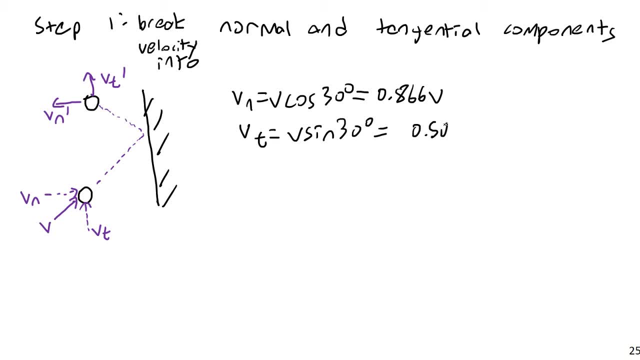 30 degrees equals 0.500 v, and I can also so step two. so let's, I have now broken down the values and I can also, so step two. I have now broken down the values and I can also so step two the initial velocity into into tangential and normal components. so step two, um realize. 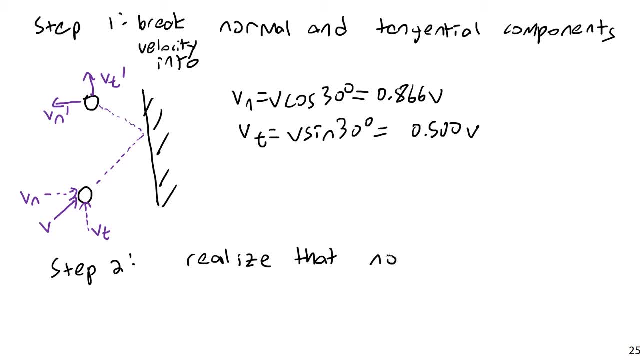 that the normal component will be conserved. so most collisions that we're going to be dealing with here, the normal component is going to be conserved. uh, is conserved, so, um, in other words, this is a frictionless law. so what do i mean by this? the normal component is going to be conserved, um, so 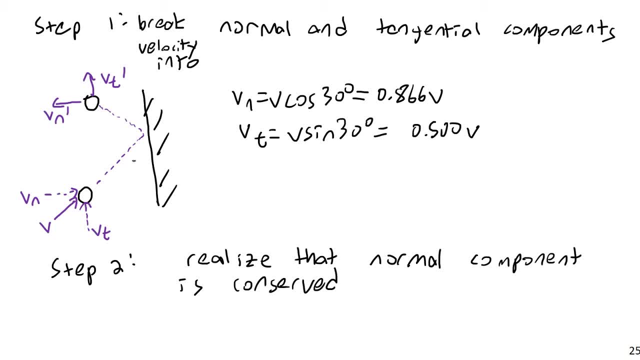 in other words, it's going to be: um, sorry, the tangential component is going to be conserved, sorry, the normal component. now we can serve the tangential component. we can start with that, the normal sort of. so the tangential component is conserved, and the reason for that is: this is a frictionless wall. 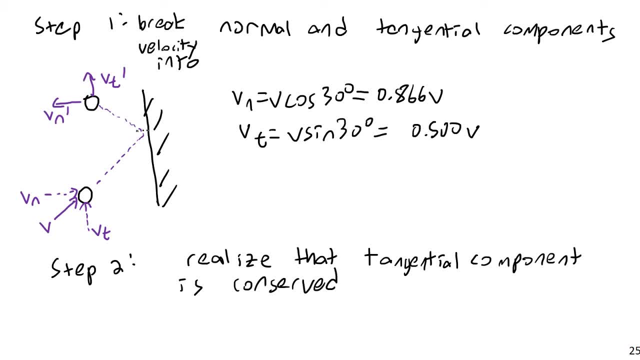 so it cannot. it can exert a force, um, in the x direction, but it cannot exert a force in the y direction. it is a frictionless wall. so there can be a horizontal exchange or a normal exchange momentum between the wall here and the ball, but there can't be any tangential exchange. 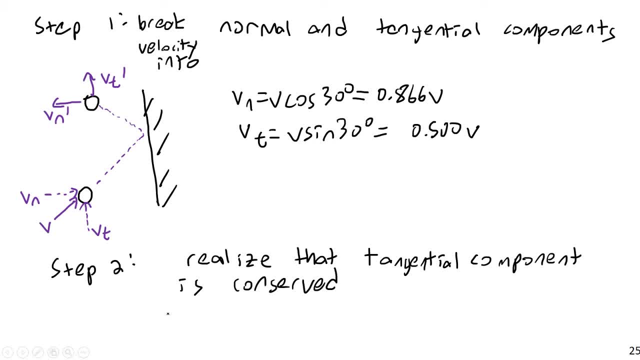 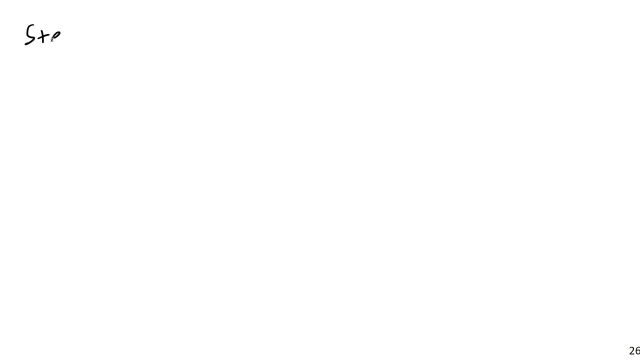 it's going to simply slide off. so from this i can say that vt prime equals vt, or will be simply equal to 0.500 times v. and then step three: i am going to apply the coefficient of restitution. the coefficient of restitution, of restitution, uh, let's see. 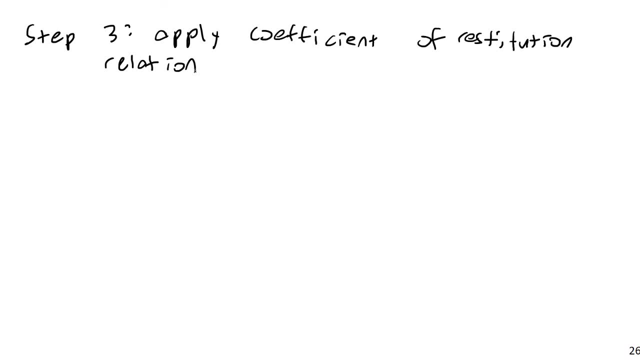 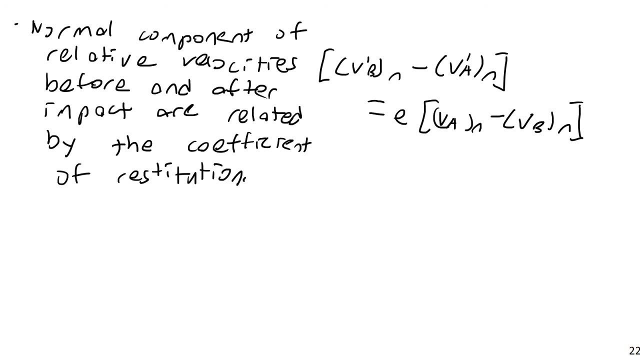 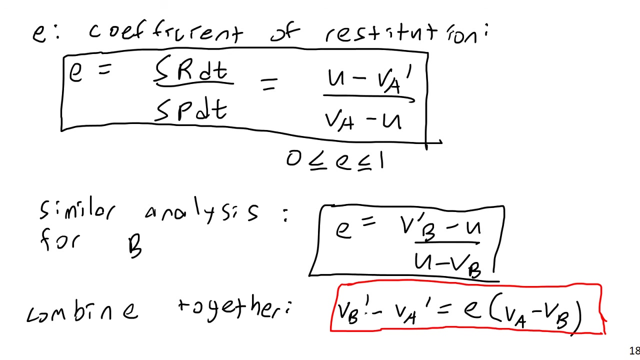 um, now, at first you might see if you're, if you're looking at the formula for coefficient restitution, you might say: wait a minute, what? how are we going to do this? okay, so i go back to the, where i defined the coefficient restitution. i have this b here. so how in the world is that going to? 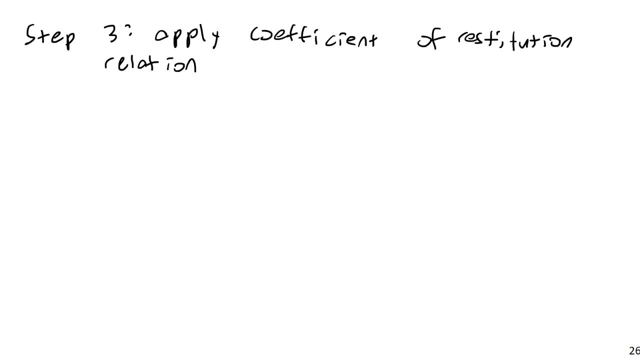 work. well, in this case we're going to treat the wall as an immovable object. so i will say: apply the coefficient of restitution relationship and then apply the coefficient of restitution relationship, uh, with zero wall velocity, with zero wall um velocity. so in other words, zero minus vn. we're doing this in the normal direction. 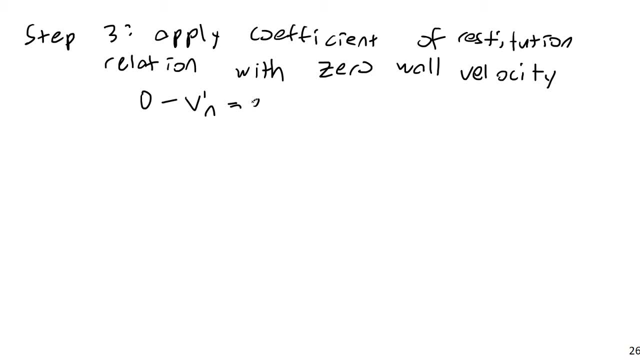 so zero minus vn prime equals e times vn minus zero. so that will go away. and so then simply uh, vn prime the normal, the final component of the final normal component of the final velocity, is going to be equal to 0.9 times vn, or just um 0 negative 0.9 times 0.866 v. 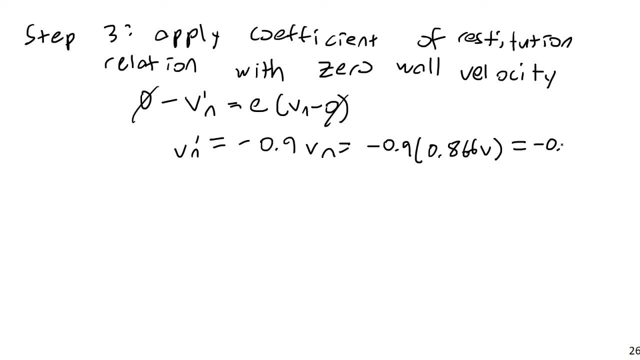 or negative, 0.779 v times v, and that would be our final component there. so i can then say that v vector compared to the initial one, v- i'm sorry, v prime vector is going to be 0.779 v times lambda n, which is the normal vector direction. 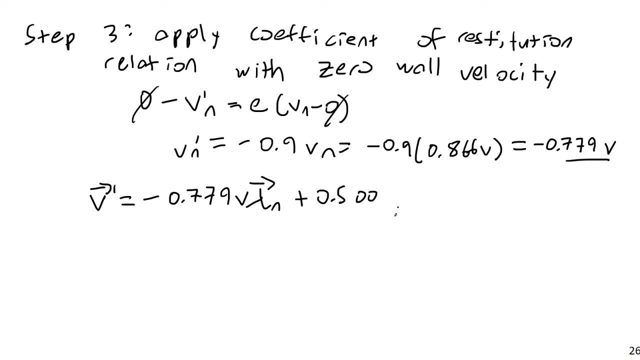 plus 0.500 v times lambda t, the unit vector in the tangential direction, or i could, if i wanted to. if i did a pythagorean on these two or found the magnitude of these, i could say that v prime is equal to 0.926 b, and I could actually find the angle here by saying the by. 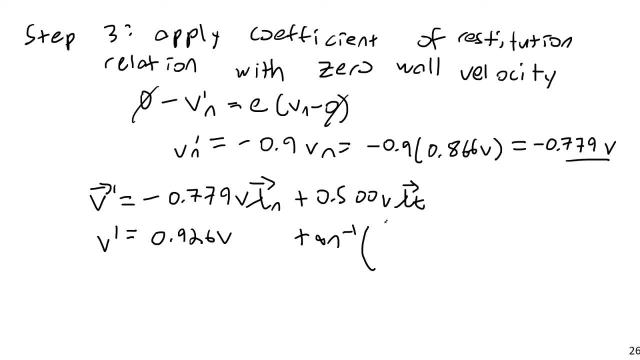 applying the inverse tangent to find the angle 0.779 over 0.500, or this would be 32.7 degrees. 32.7 degrees. so this is our magnitude, or this is our magnitude, and this is our direction, or this is it in rectangular vector form. okay, so maybe. 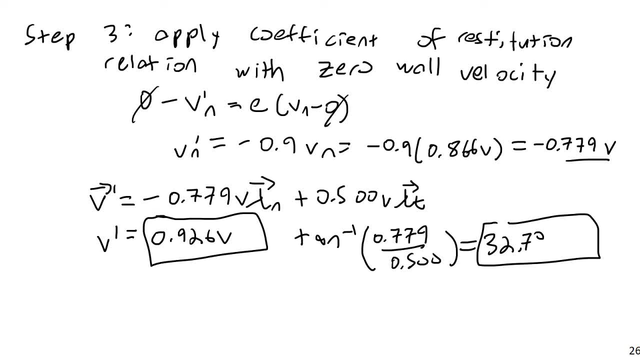 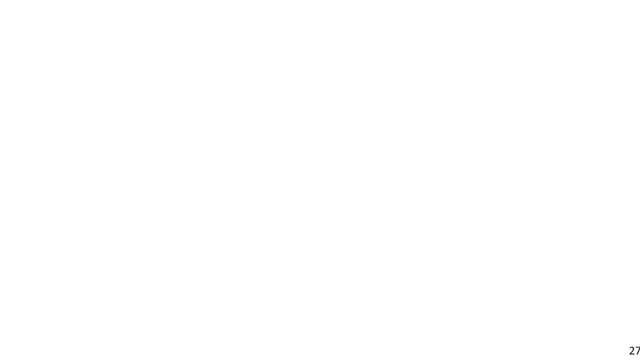 I'll work through one more example, this time looking at the collision of two particles moving in oblique impact in two directions. this here, let's say, I have something like this: this is going to be an oblique impact. this is going to be an oblique impact. 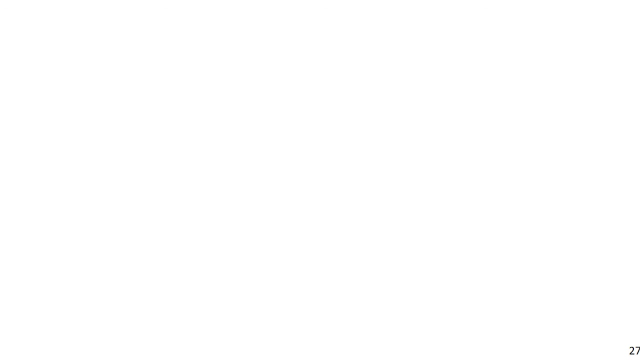 of two different masses, each with their own initial velocity. so let's work through this. so consider two spheres or two point particles colliding at a point. this is going to be a lot of collision. I'm going to construct this. usually it's good to for doing a problem like this. your first. 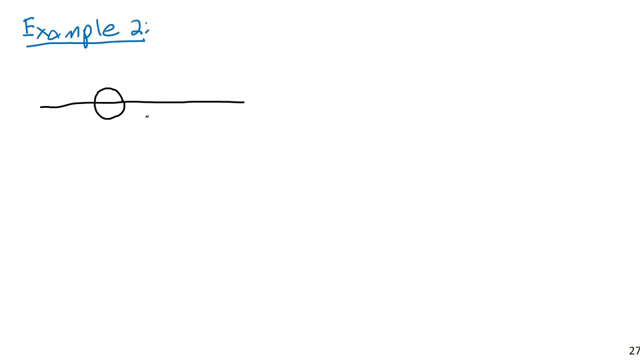 strategy should be to resolve it into normal tangential components. so if you notice, what I'm doing is I'm actually. this didn't necessarily have to be along this. initially it could have been something at an angle like this, but what I've done is I have redrawn it and redone the math and run through trigonometry to 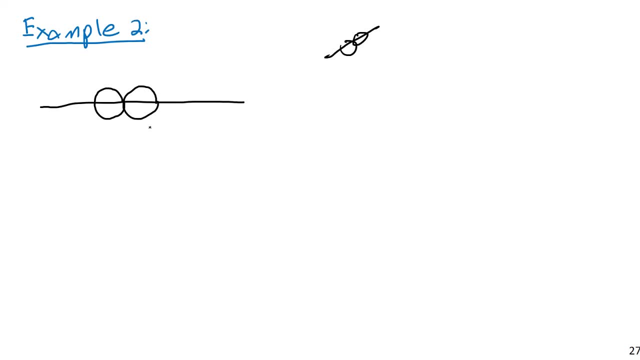 find angles relative to the, relative to the thing here, relative to things, sorry- relative to the line of impact. this is the line of impact and, um, each of these is going to have a mass M. so this is given here, all of this is given. so I have two spheres, each with the same mass. 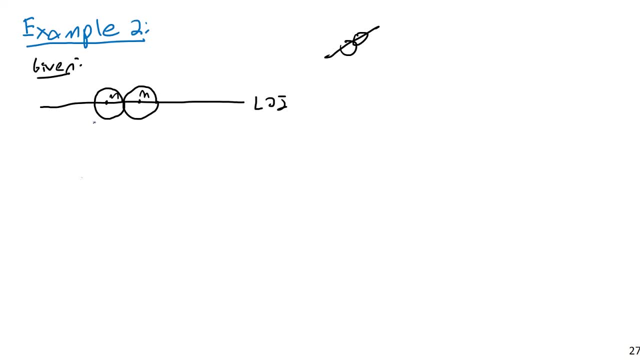 and this one will have a VA of 30 feet per second and VB here, so they'll have the same mass of different velocities. VB is 40 feet per second, 40 feet per second and the angles here. well, this one will be an angle of 30 degrees and this 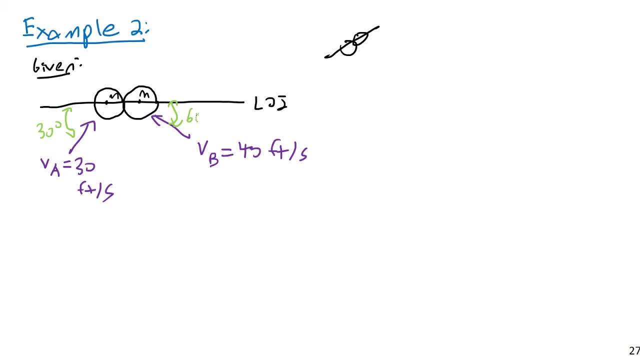 one will be at an angle of 60 degrees. okay, so all this is given. and also they are, they're going to collide without friction and the masses are the same, and also E is going to be equal to 0.9. and so, all this is given, I wish to find, oh, the magnitude and direction of the final. 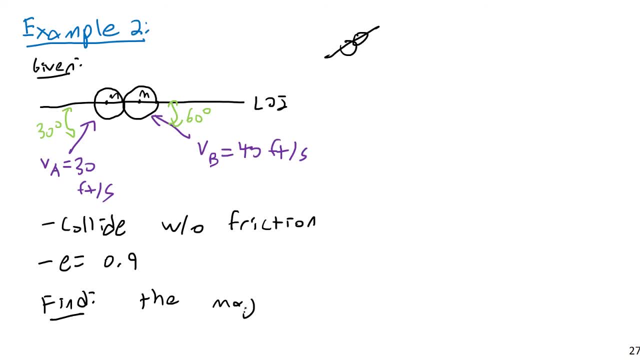 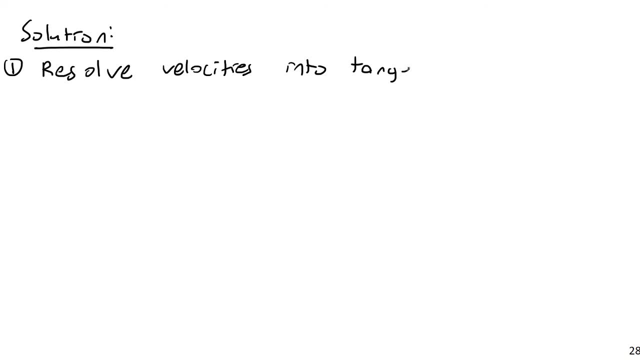 one one. resolve the velocities into one one. resolve the velocities into tangential and normal components and tangential and normal components and tangential and normal components and normal components. so VA normal is going. normal is going to equal to VA cosine 3.5.. normal is going to equal to VA cosine 3.5.. 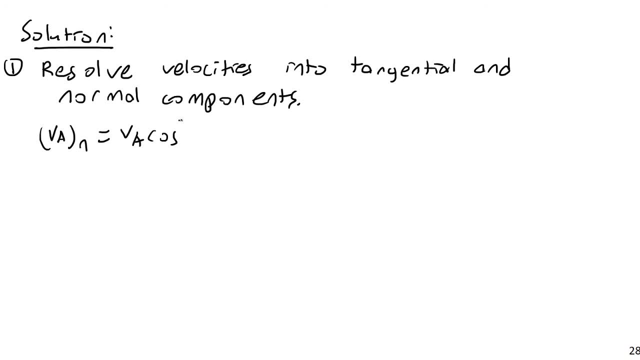 normal is going to equal to VA cosine 3.5.. VA cosine- theta- VA cosine 30 degrees. which VA cosine theta VA cosine 30 degrees. which VA cosine theta VA cosine 30 degrees, which will be equal to 26.0 feet per second. 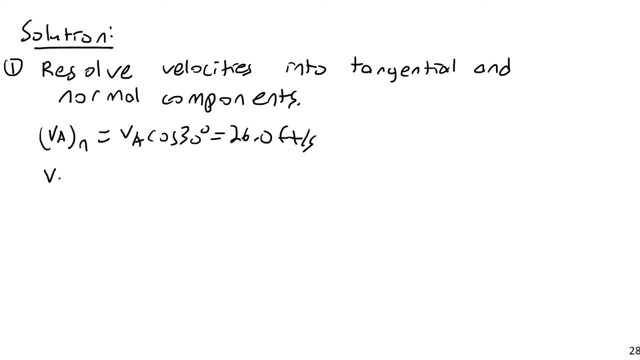 will be equal to 26.0 feet per second will be equal to 26.0 feet per second. VA tangential tangential will be equal to VA tangential tangential will be equal to VA tangential tangential will be equal to VA sine of 30 degrees, which will be 15. 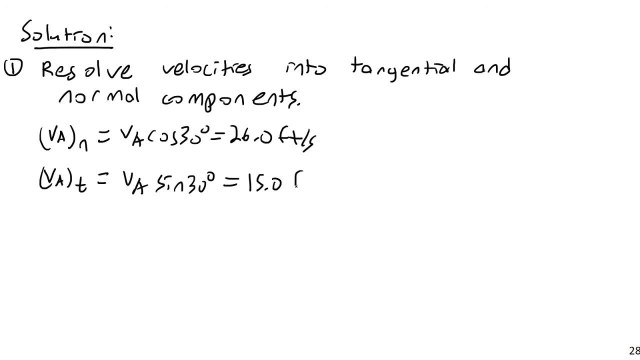 VA sine of 30 degrees, which will be 15. VA sine of 30 degrees, which will be 15 feet per second. feet per second, feet per second. and then VB normal will be equal to, and then VB normal will be equal to, and then VB normal will be equal to: negative VB cosine: 60. negative VB cosine. 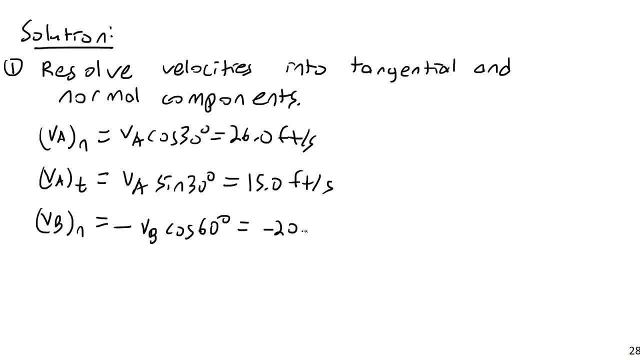 negative VB cosine: 60. negative VB cosine. negative VB cosine: 60. negative VB cosine: 60 degrees is equal to negative 20.0 feet. 60 degrees is equal to negative 20.0 feet. 60 degrees is equal to negative 20.0 feet per second. and VB: tangential or 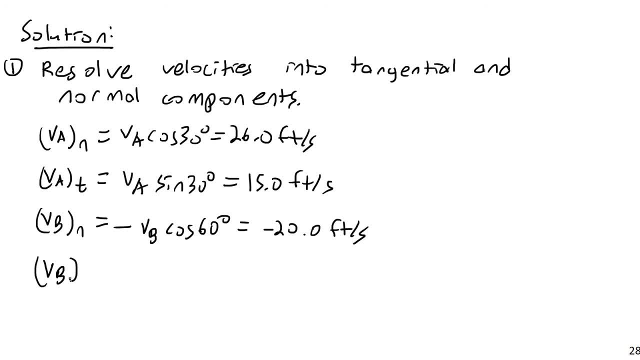 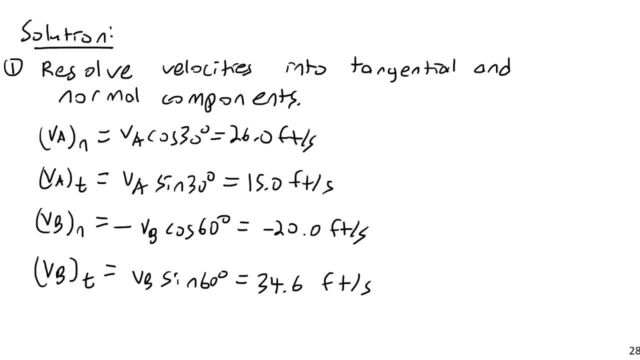 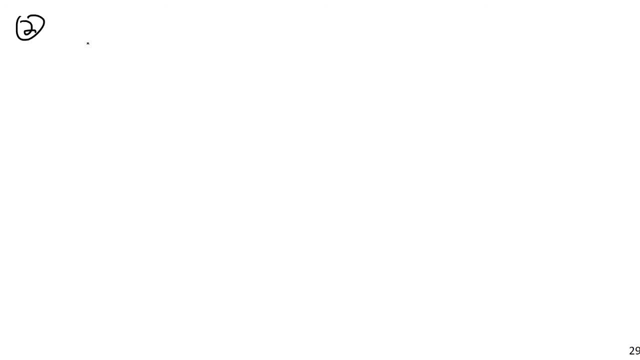 tangential VB normal is equal to negative. 20.0 feet per second. and VB tangential or tangential value of VB NiceR. tangential VB- normal is equal to negative. 26 is equal to negative. 27 is tangential VB normal is equal to negative. 27 is equal to negative. 27 is beautiful. 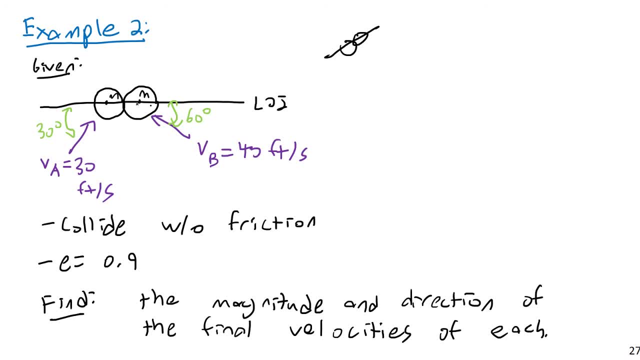 to collide and each of them has a normal component and a tangential component. So they can exert forces on each other in the normal direction, here, along this plane, along this line, but they cannot exert any force along each other in this line. So therefore, the tangential basically along this. 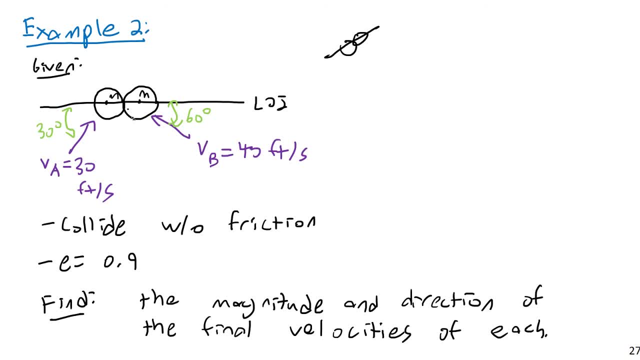 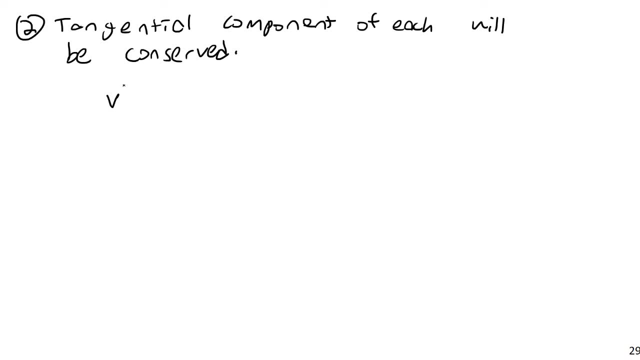 direction, the vertical direction is drawn here- their velocities will be unchanged. Each one individually, their velocities will be unchanged. So in other words, V prime A, the tangential component, is going to be equal. so the final one is going to be equal to VA tangential component and VB prime. 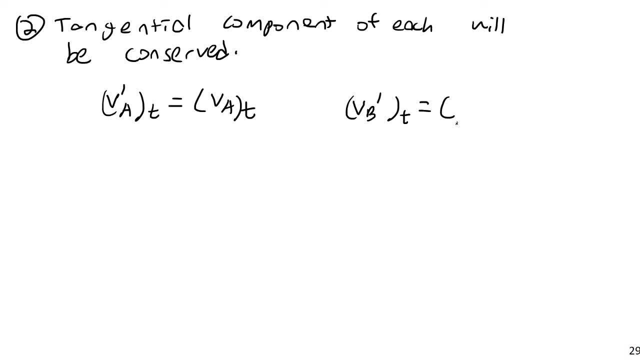 tangential component is going to e, equal to VB tangential component, and this is equal to 15.0 feet per second. So I already know the tangential component of VA, prime A. Okay, I think we have tested this so far. it would just be less than 3ppa squared in three complication. 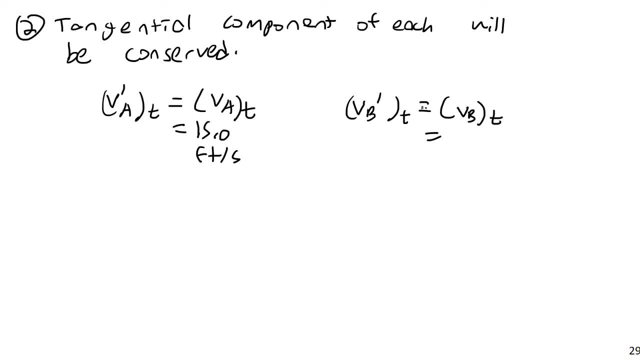 So I have how to correct that and say each one has 1pi and 4pi and 6p and and the same one for VB, prime, 34.6 feet per second here. so step 3, I apply another relationship and that is that the total normal component normal. 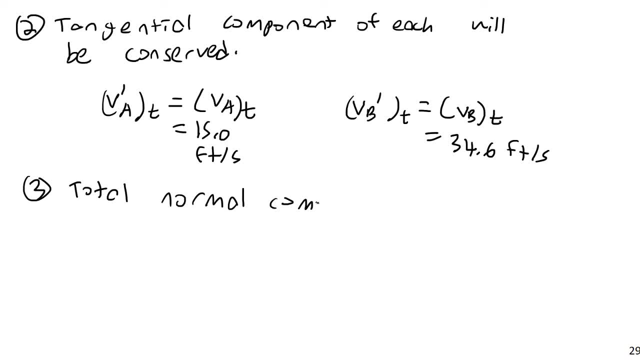 component of the momentum of the two-ball system is conserved. all right. so let's see here: MA, VA, normal normal component. MA times the mass of A, times the normal component of A's initial velocity, plus MB, VBN, the normal component of ball B's initial velocity equals- and notice I'm using, I'm 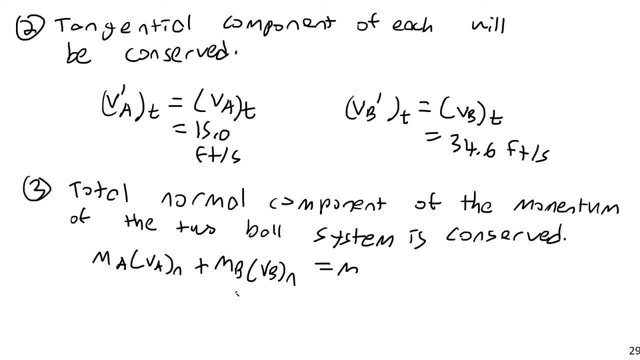 labeling these as separate masses. but and so if these weren't the same mass, you would need to use different numbers, different values. but in our case we can, actually will be able to replace these both with a single M, so MA V- prime a in the normal direction, plus MB V- prime B. 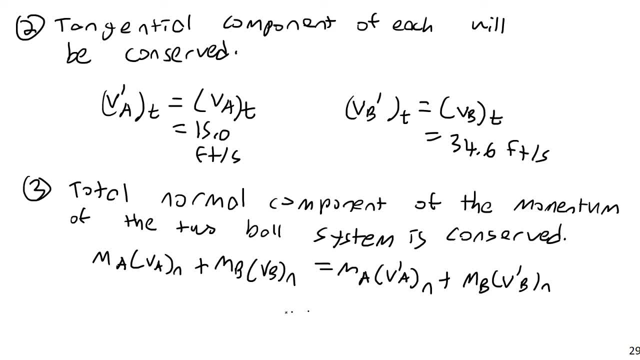 in the normal direction. and I can replace these all with m here and I can also put in the initial velocities. so M 26 m plus M negative 20 is equal to V prime A- normal times. M plus V prime B- normal component. This is the normal component. Let me put the M's first because that will be a little bit neater. 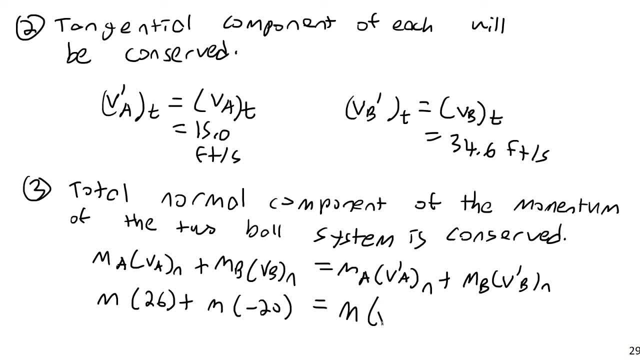 M times V prime A normal plus M times V prime B normal. or here I could divide all the way across by M. so I could also say that if I divide all the way across by M I get that the normal components of the two final velocities of the following relationship: V A prime N plus V B prime N. 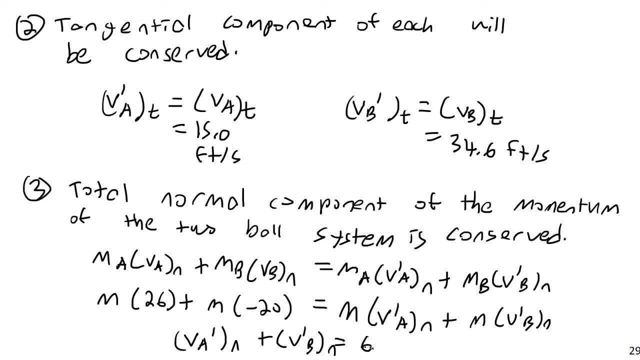 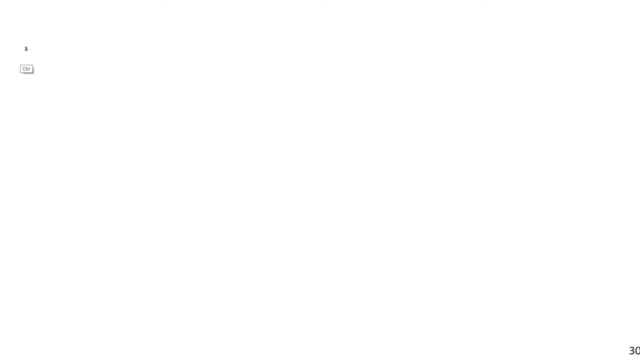 will simply be equal to 6.0.. Will simply be equal to 6.0. and then another relationship I can apply. oh, we skipped four a bit. Another relationship I can apply for here is that the normal relative velocities of each are governed by the coefficient of restitution. 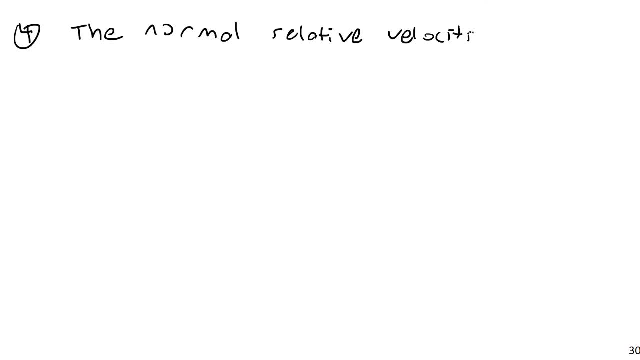 Of each are governed by the coefficient of restitution, By the coefficient of restitution Of each are governed by the coefficient of restitution. So in other words, V prime A minus V prime B, normal component of each is equal to E, our coefficient of restitution, E not Euler's number. the coefficient of restitution is equal to V A, normal minus V B, but only the normal components of these. These aren't the total velocities, only the normal components of these. 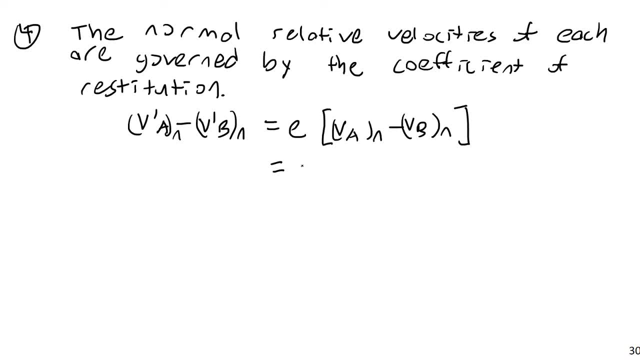 These aren't the total velocities, only the normal components of these. So this is equal to 0.9 times 26.0 minus negative 20.. So do pay attention to directions here- and that equals 41.4.. So in other words, I know that the difference between these two is simply 41.4.. 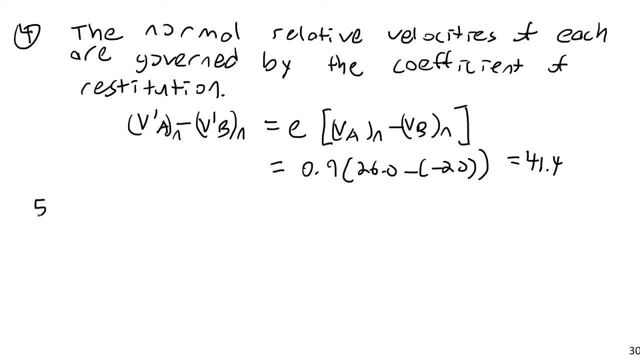 So if I solve equations, so step 5. Solve equations from 4 and 3. A system of simple linear equations, not that bad, Actually. let me rewrite this so it's very clear: V prime A, normal minus V prime B, the normal component is going to be equal to 41.4.. 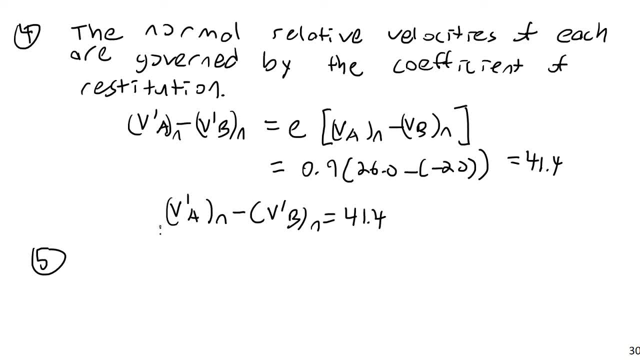 And then finally part 5. here I will resolve. I will apply a balance of equations, So solve the solve equations from parts 3 and 4 and 4 together and we can get that. if you do that you'll get that V prime A, the normal component, is equal to negative 17.7 feet per. 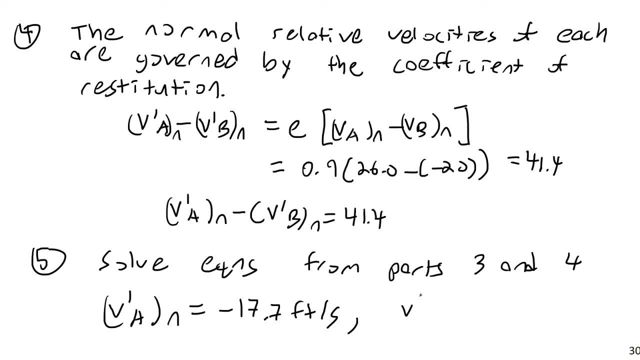 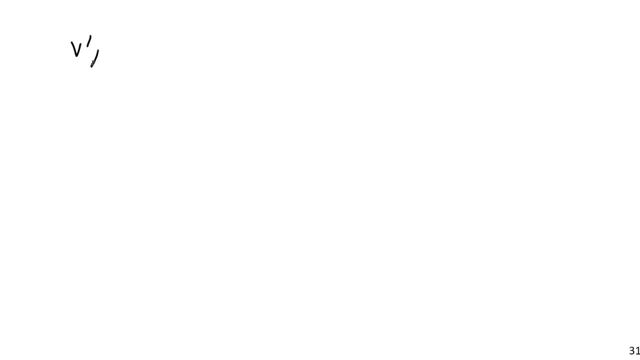 second, And that V prime B, The normal component, is equal to 23.7 feet per second here. And so if I were then to summarize all of this, I would get that V prime A is equal to negative 17.7 times lambda t, the tangential component of a tangential unit, vector plus: 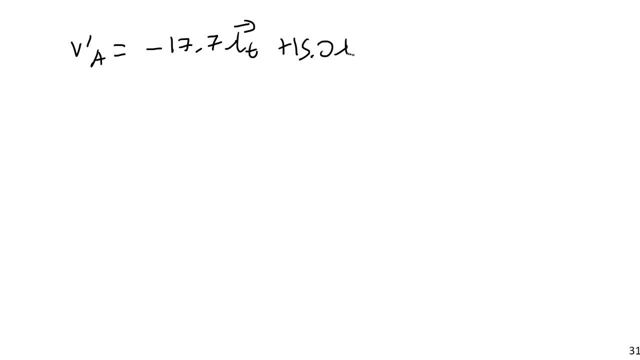 15.0 lambda n, The normal of the unit vector in the normal direction. Or I could say if I looked at magnitude, and if I want to look at magnitude and direction, I could say V prime A equals 23.2 feet per second. 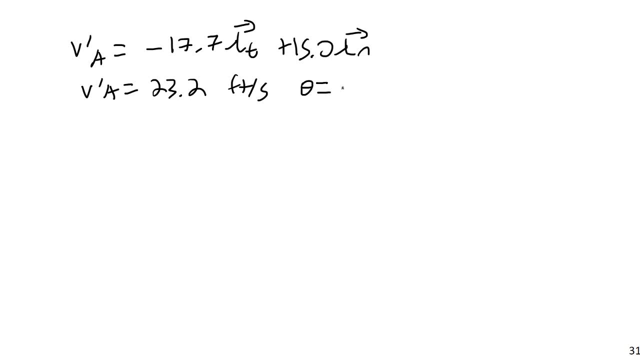 And that the theta by doing a angle an inverse tangent is equal to 40.3 degrees. And I could also say that the V prime B Is equal to 23.7 times lambda t And that the theta by doing a angle an inverse tangent is equal to 40.3 degrees. 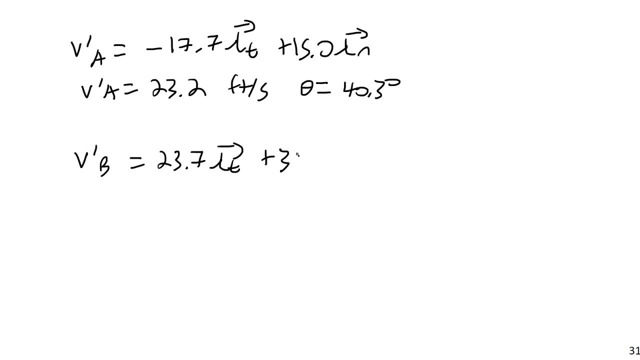 And I could also say that the V prime B Is equal to 23.7 times lambda t Plus 34.6 times lambda n unit vector. And then, finally, if I wanted to put this in magnitude and direction notation or radial form, it would be 41.9 feet per second. at an angle of theta equals 55.6 degrees. 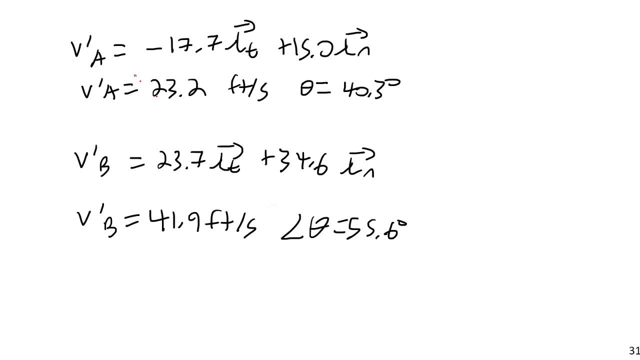 And that would be my final answer here. So that will conclude my examples here. I just want to thank you for watching. I'll see you next time. Bye, Bye, Bye, Bye, Bye. I just wanted to work through a couple brief examples to finish up part three of this lecture over collisions, impulse momentum, etc. 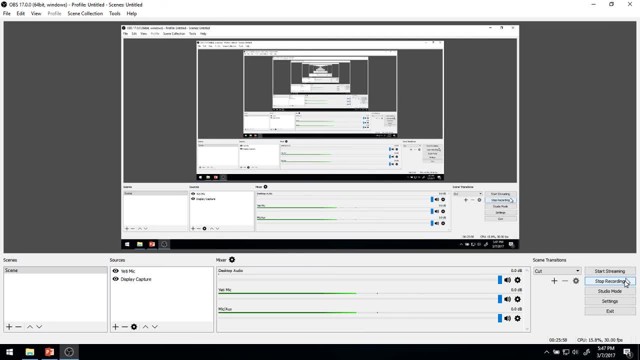 So that will do it for today. Thank you for watching And, as always, thanks.